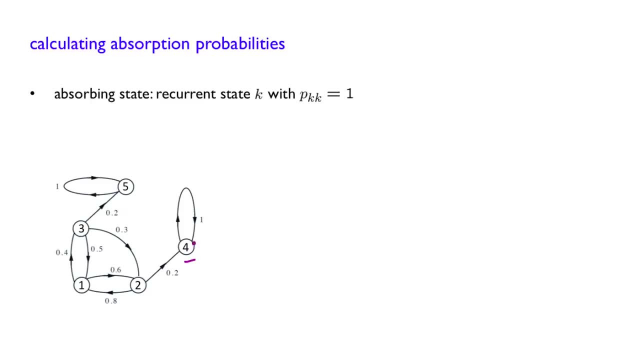 First, it seems plausible that this probability of ending in 4 will depend on where you started. If you start in 2, you probably have more chances of getting to 4 than if you started from 3.. Because, Yes, Why? 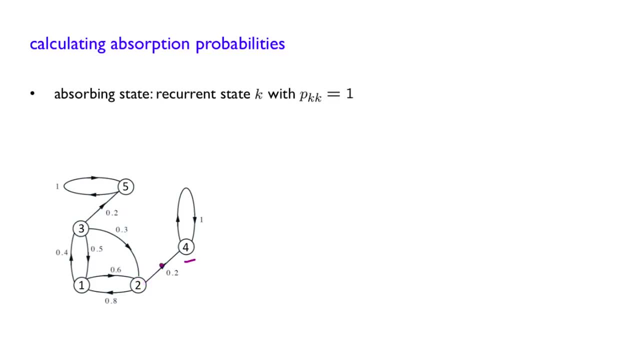 Why? Because if you start from 2, at the next step you have immediately the chance of getting to 4.. But if you start from 3, there is some chance that you will go to 5 and never go to 4.. 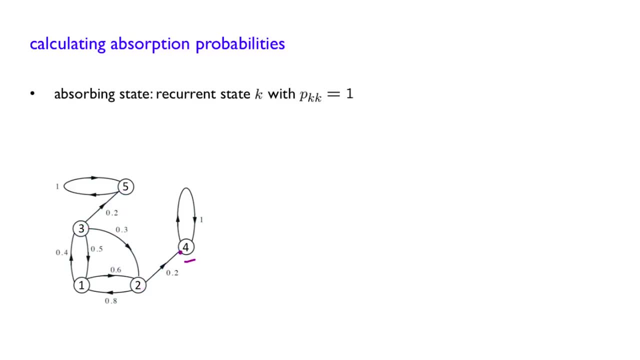 Or you will have to go through 2 in order to get to 4 anyway. So it looks like the probability of reaching 4, given you started from 2, will be bigger than if you started from 3.. Now, from 1,, it's unclear. 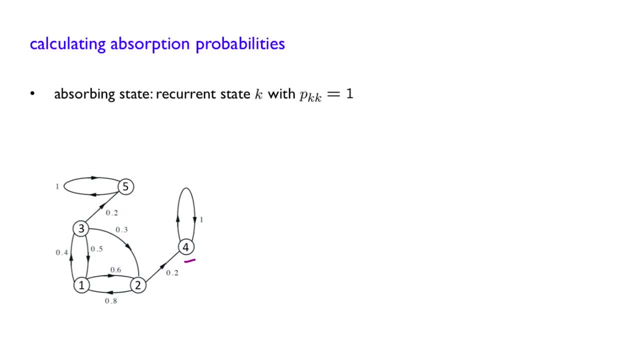 Let us be systematic, then Let us consider all possible probabilities that you end up in 4, depending on the initial state. So let us ask this question: What is the probability a of i that the chain eventually settles in 4,, given that it started in i? 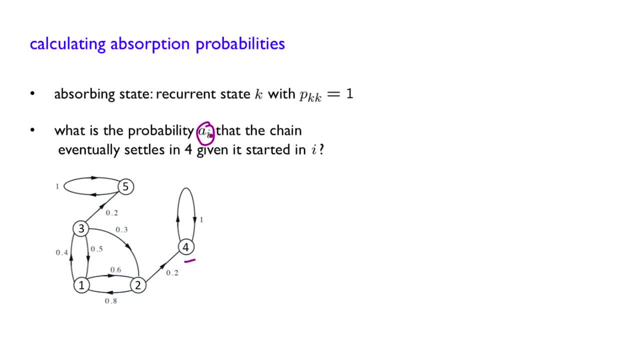 So, in other words, a of i is the probability that you end up in 4,, given that you started in i. Now the answer to that question is very easy. for some cases, If you start in 4, the probability that you end up. 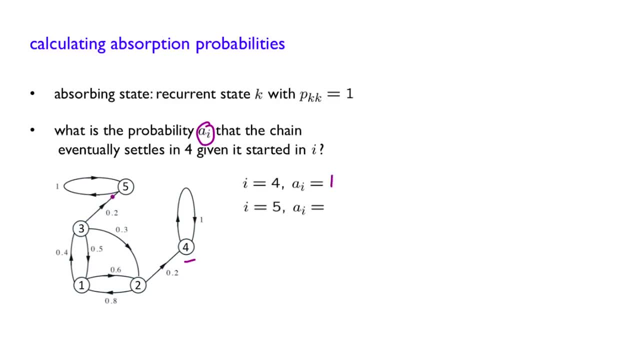 in 4 is 1.. And if you start in 5, the probability that you end up in 4 is 0. There is no way that you can go from 5 to 4.. What about the other cases? Well, it's not so clear. 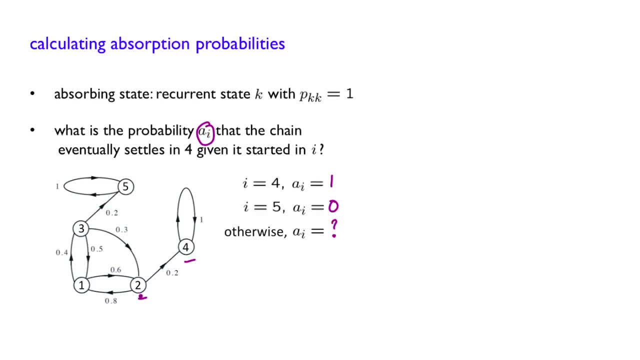 Let us consider, for example, that you started from 2.. What could happen next? Well, from state 2,, let's build a tree. You can either, with a probability 0.2,, go to 4, or, with a probability 0.8,, go to 3.. 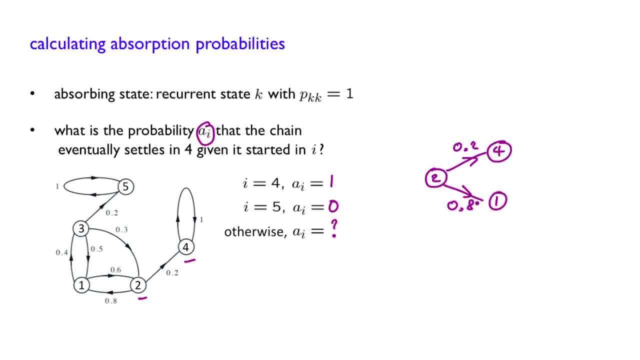 OK, Let's go to 3.. Let's go to 3.. Let's go to 3.. You will go to 1.. Now, in the first case, you're done, You reach 4.. But in the second case, you arrive in 1.. 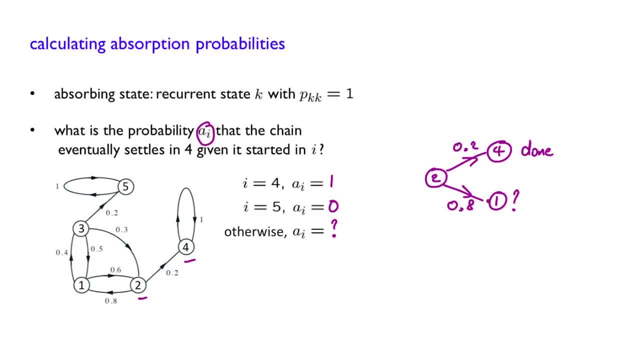 And what happened next? You don't know. But what you know is that, from that state, either, eventually you go and get trapped in 5, or you go and eventually get trapped in 4.. What are the probabilities of these events? Well, we don't know. 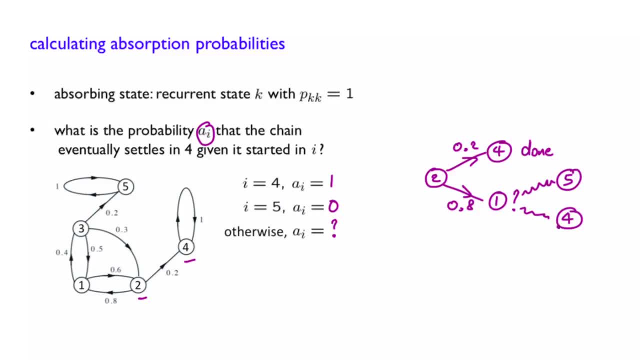 But one of them has been defined, which is the probability of ending up in 4,, given that you started in 1.. And that has been defined here. This is nothing else than a1.. So the overall probability of interest for us, which is a of 2,. 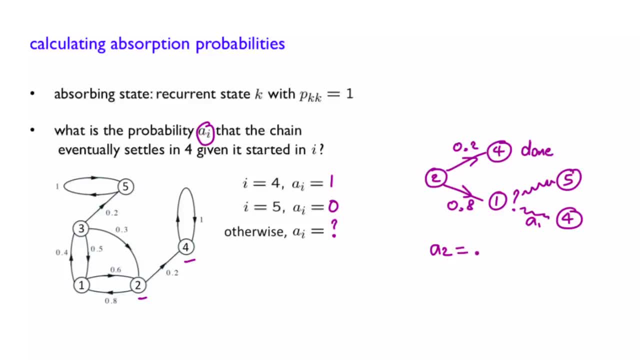 using the total probability theorem, you can enumerate all options. It's: with probability 0.2, you will go to 4.. And then the probability of going to 4, given that you started in 4, is a4.. Plus 0.8 times a1.. 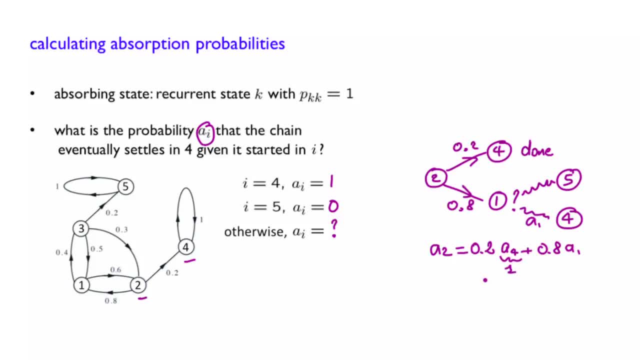 Now, a of 4 is, of course, 1, as we have discussed before. So we get the relation between a2 and a of 1.. Now, of course, you can do the same thing for the other state. For example, if you started from 1, what can happen next? 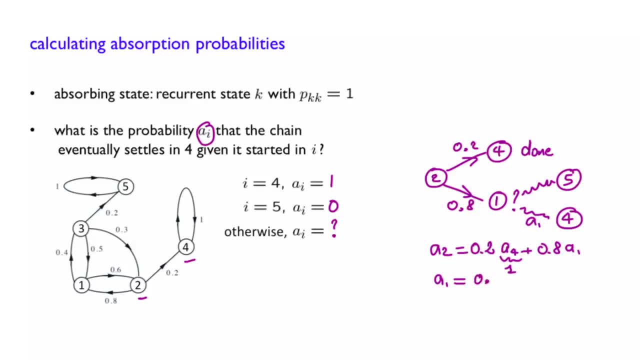 Well, you can go to 2 with a probability 0.6.. Once you're in 2, you are asking yourself what is the probability of reaching? Well, by definition, it's a2.. Or from 1, you go to 3, with a probability 0.4.. 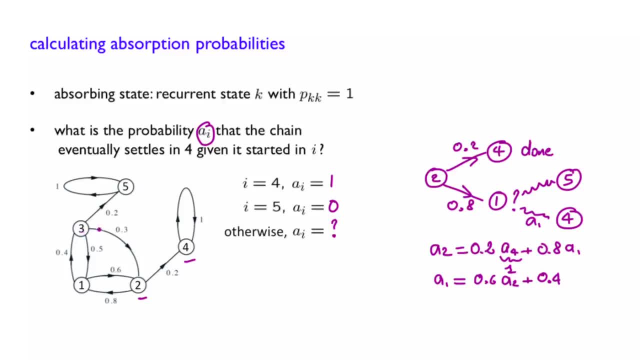 And given that you have done that, what is the probability that eventually you reach 4? It's a3.. If initially you start with a3, what can happen next? Again, with a probability 0.3, you will end up in state 2.. 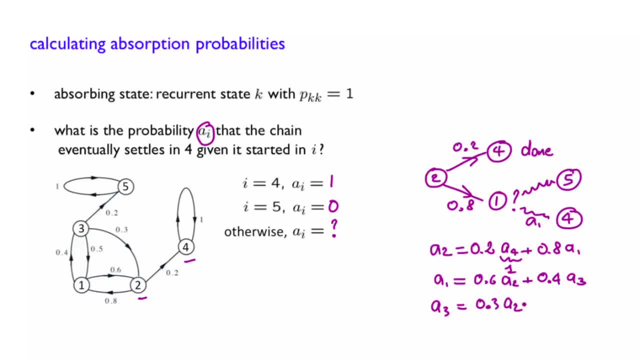 And there a of 2 is the probability of interest. Or with a probability 0.5.. 0.5, you go to state 1. And in that case you get a of 1.. And finally, with a probability 0.2, you get trapped in 5.. 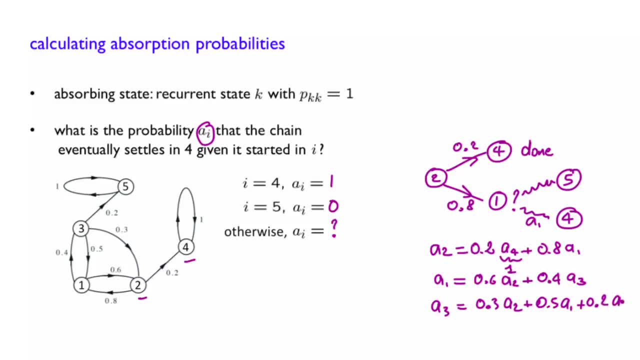 You can write it if you want, but 0.2, and you get trapped in 5.. But we know that a of 5 is 0, so this term will disappear. So in the end you get a system here. 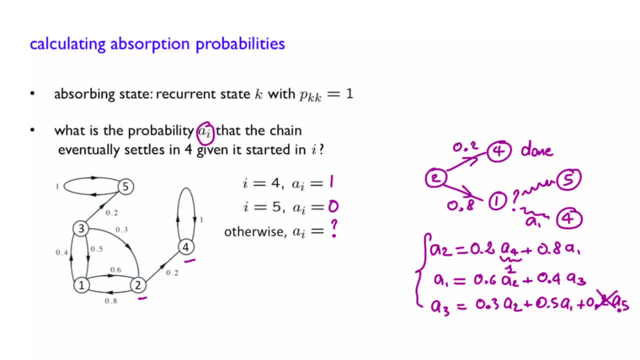 After you replace a4 by 1 and a5 by 0, you get a system of three linear equations with three unknown, And it is easy to solve. I will not do that, You can do it yourself, But here are the results. 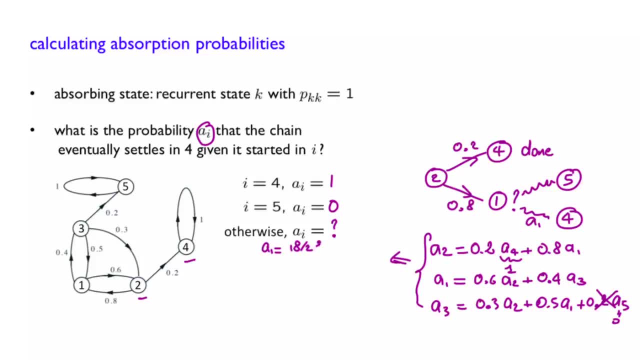 You will get. a of 1 equals 18 over 28.. a of 2 will be 20 over 28.. And a of 3 will be 15 over 28.. Now I expressed them so that we can compare them easily. 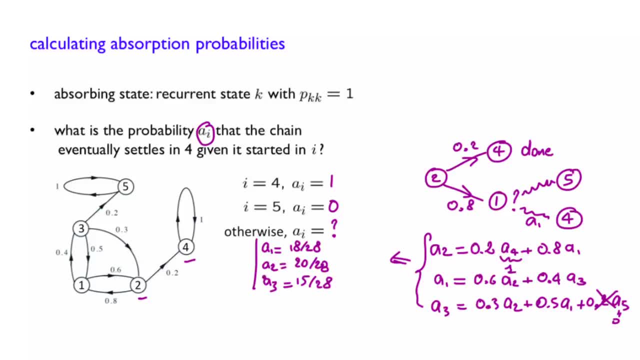 But I'm going to do it again And as a sanity check, you can verify that indeed, the probability starting from 2 will be larger than the probability starting from 3.. And it turns out that a of 1 will be in between the other two. 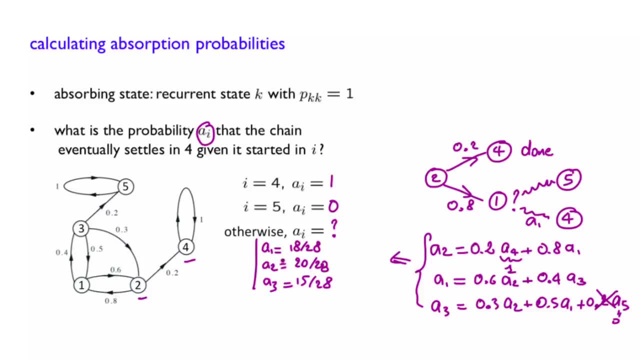 So these probabilities are consistent with our previous intuitions. As an aside, note that you could have written a system of five linear equations with five unknown, the five unknown corresponding to the five states possible. In fact, we had our five equations here. 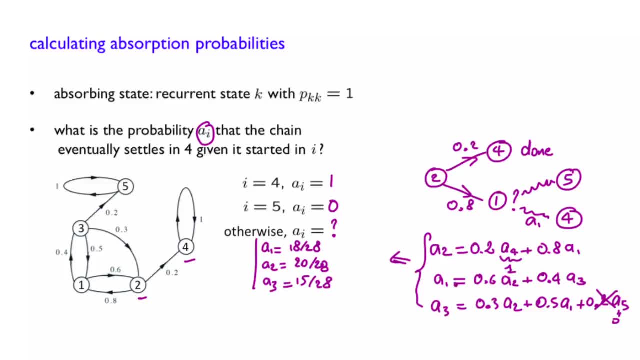 Here was 1,, another one here and 1,, 2, 3,, so 3 plus 2, 5.. Of course, this one was easy: It was a4 equals 1 and a5 equals 0. that you can replace then there. 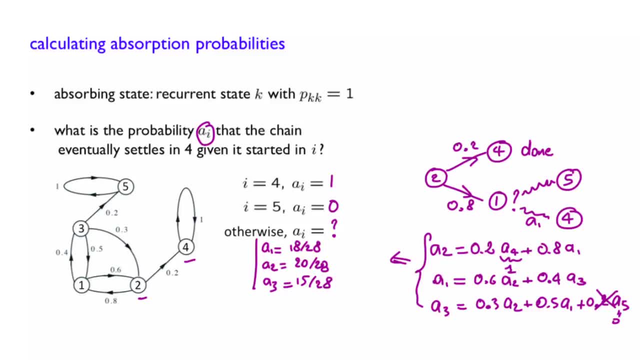 And you get a limited or restricted or smaller system of three equations with three unknown. Now what if you had been interested instead in finding the probability b of i that the chain eventually settles in 5, given you started in i? How to do that? 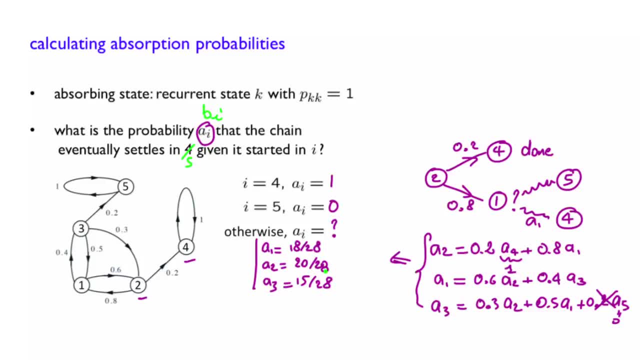 Well, you can repeat exactly all these calculations that we have done, but looking at 5 as the state of interest. But of course you don't have to do this For any state i, given that you started in i, you will eventually, with probability 1,. 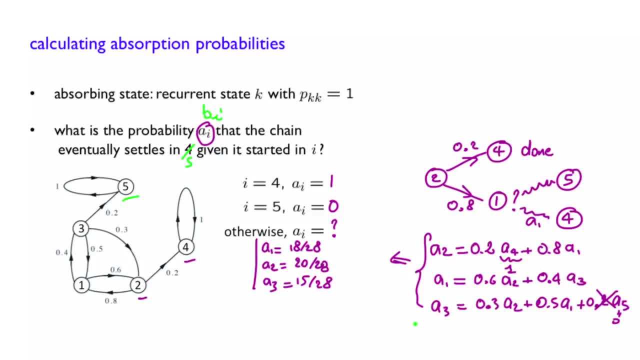 end up in either 4 or 5.. So you have a of i plus b of i equals 1 for all possible i. So once you have calculated a1, a2, a3, a4, and a5,, you get b1, b2,, b3,, b4, and b5 by using this formula.